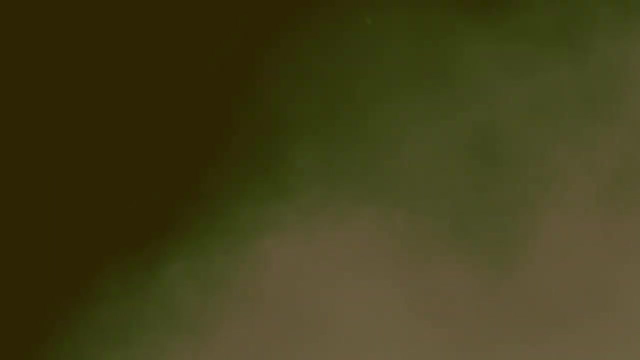 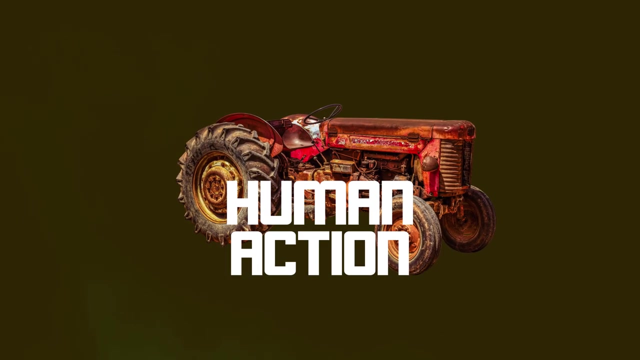 rate. Although soil degradation can be caused by a number of natural factors, increasingly soil quality is affected by human actions. Today, I'm going to narrow in on one of the bigger human caused factors- industrial agriculture- in order to answer what soil degradation is. 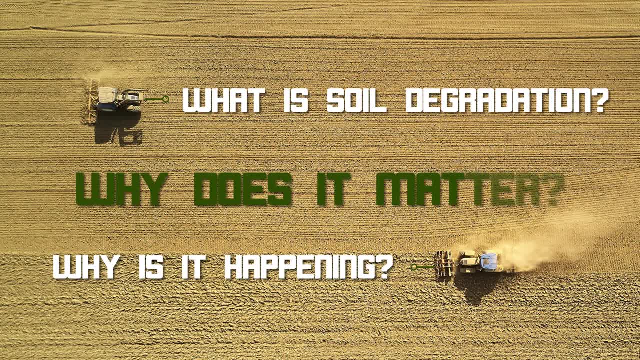 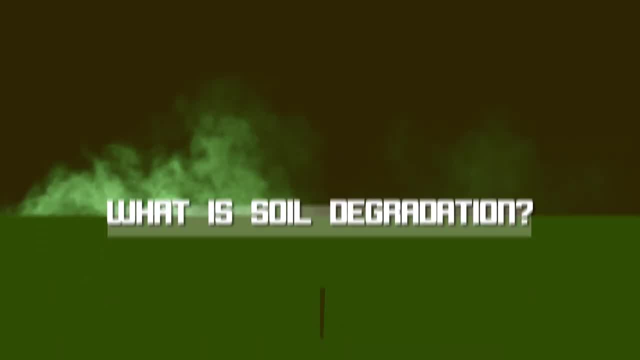 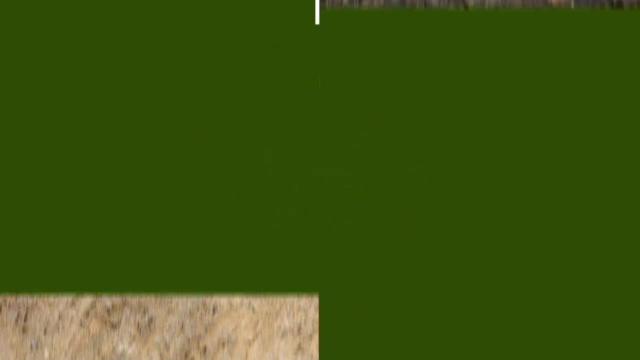 why it's happening and why we need to strive for better soil health. So first, what is soil degradation? Quite simply, it means a decline in soil health as a result of misuse or poor management. Soil can vary widely in its depth depending on whether it's young or stable and old. 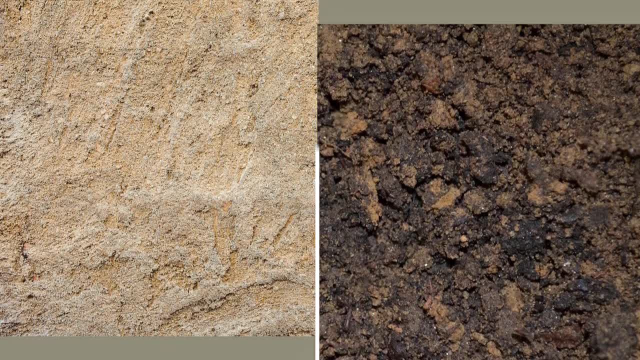 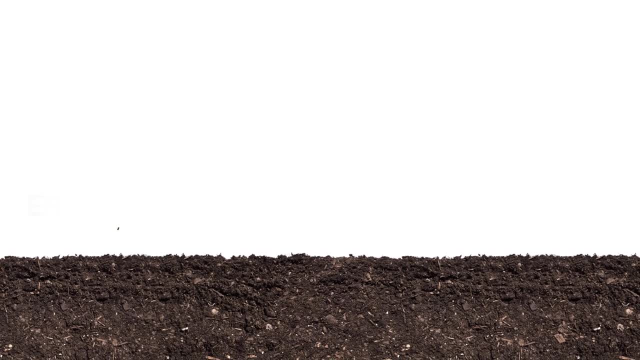 but it's generally teeming with life. According to the Earth Institute at Columbia University, it's estimated that an acre of soil may contain 900 pounds of earthworms, 2,400 pounds of fungi, 1,500 pounds of bacteria and a little over a quarter of a pound of soil. So it's a very 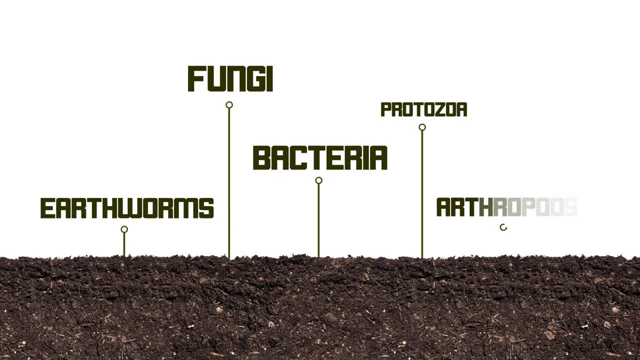 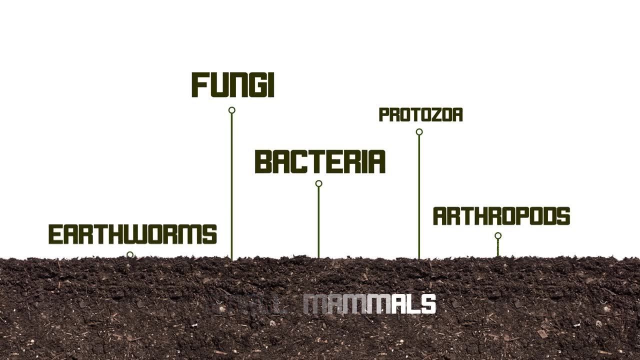 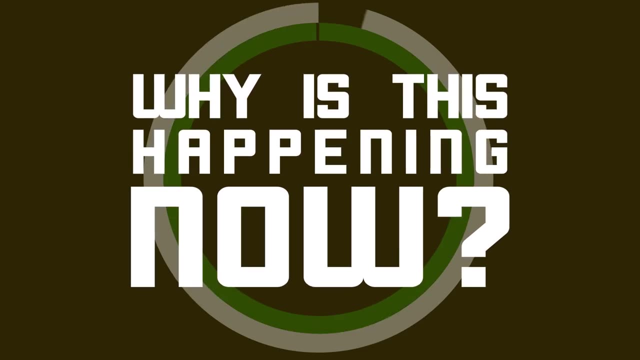 small area 133 pounds of protozoa, 890 pounds of arthropods and algae, and even, sometimes, small mammals. And when soil health is affected, this biodiverse system wanes. Why, then, is soil degradation such a big issue now, While the quality of topsoil can definitely be damaged? 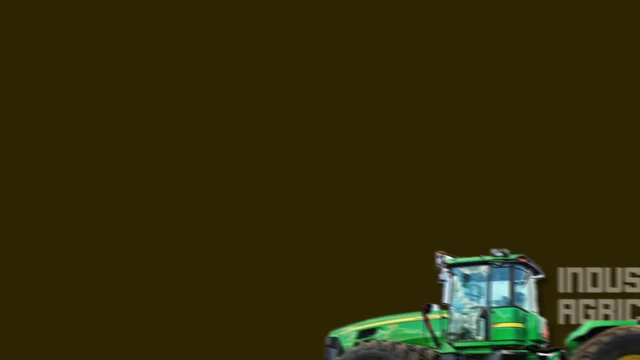 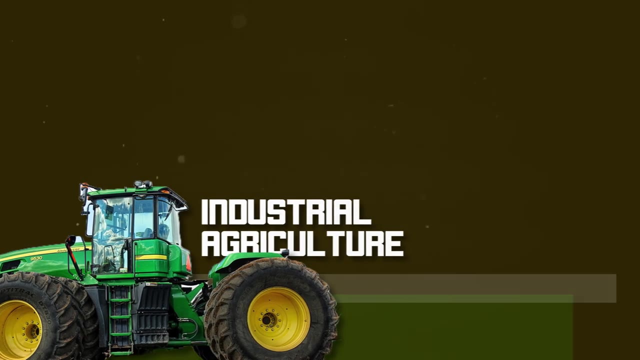 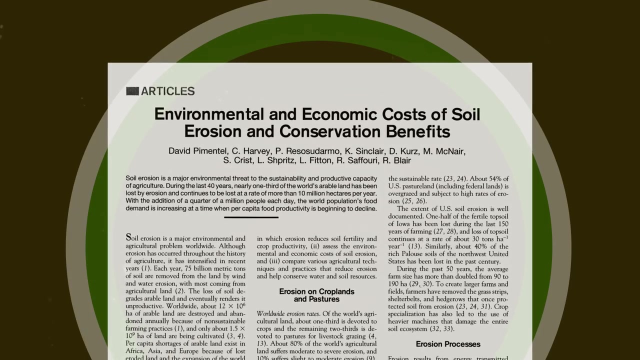 by natural occurrences like floods or wind. the rate of topsoil loss has increased radically over the last 200 years in the United States as a result of modern agricultural problems. In Pimentel et al's study on the economics of soil erosion and conservation, they estimate that 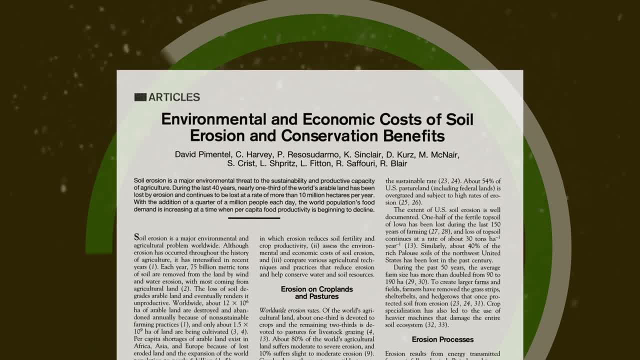 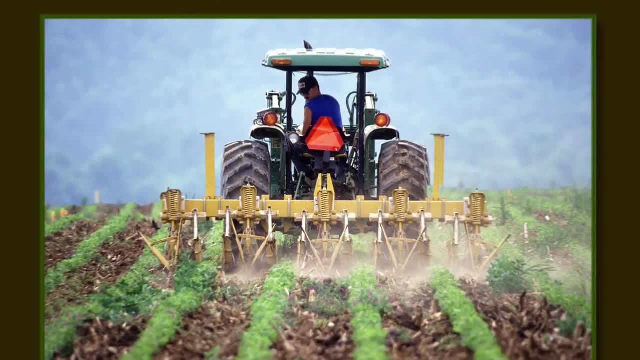 in the United States, soil has been lost at about 17 times the rate at which it's formed. We can pin some of this soil loss to the intensive cultivation practices and monocropping of industrial agriculture. When we till and turn over a field for the next season's crop, using 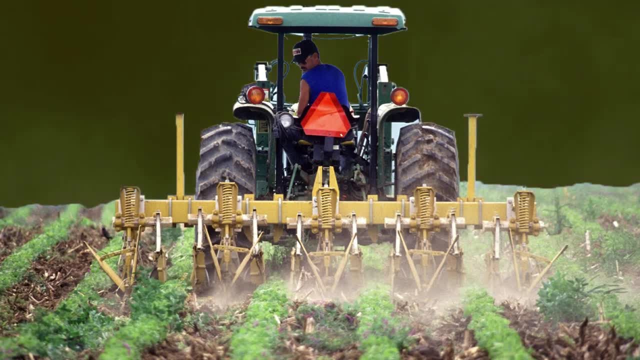 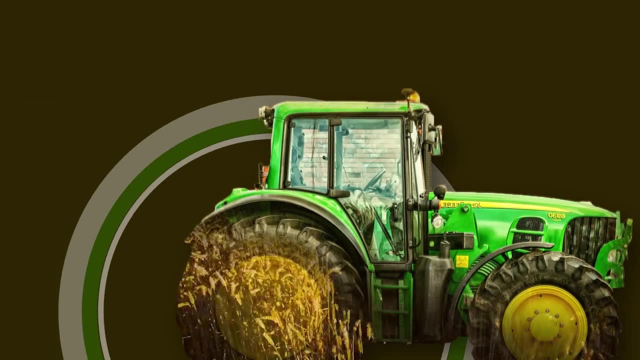 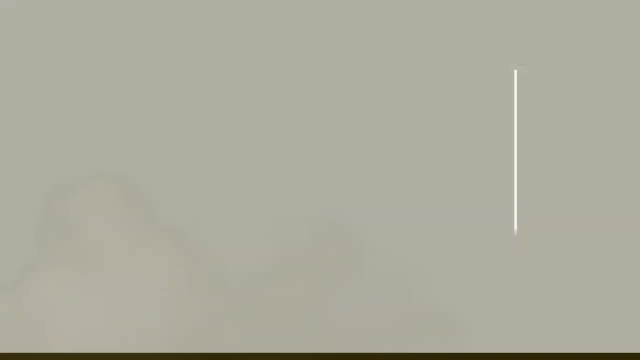 large combines, the topsoil is decimated. Much in the same way, habitat is lost. when clear-cutting a forest, Tillage aerates the soil by breaking up its composition, but in the process compacts the soil underneath and kills the wealth of microorganisms hidden to the naked eye. As 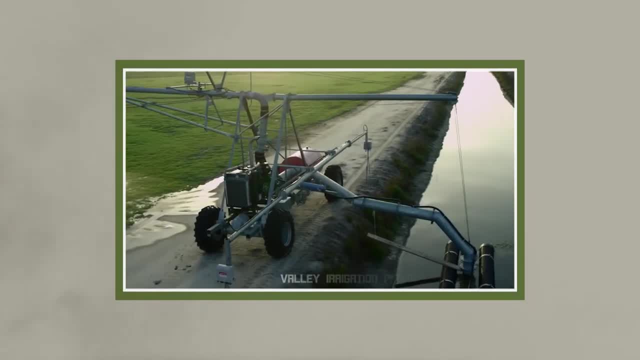 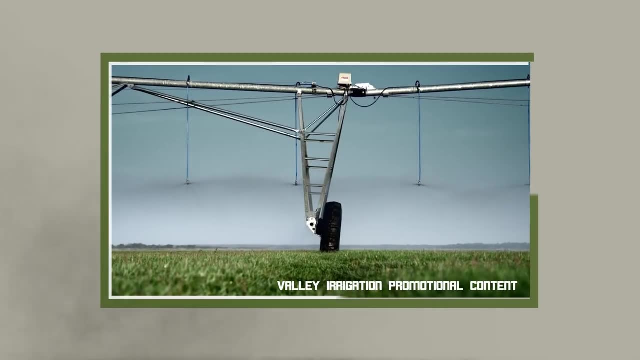 a result of many years of industrial cultivation practices, the topsoil lies void of life and then needs to be injected with nutrient-filled fertilizer and chemicals, which in turn alter the chemical makeup of the soil and make it even harder for essential organisms to survive. 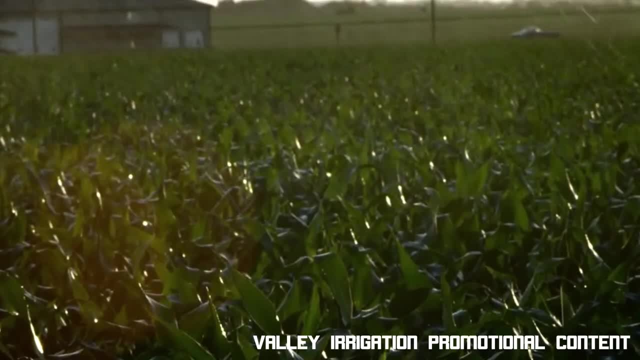 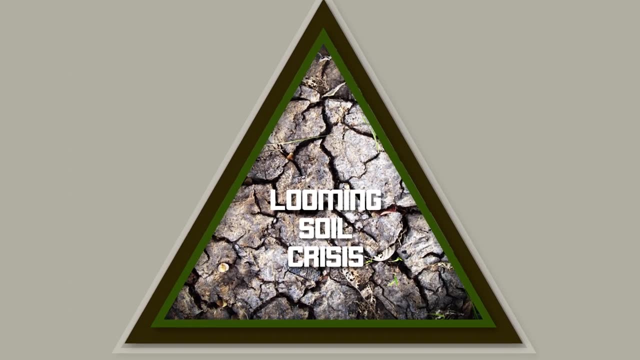 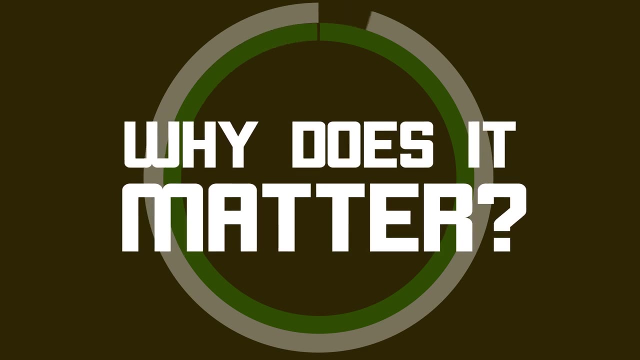 In short, cultivating the soil always results in the decline of its fertility and health, And the continual use of intensive cultivation over the last century has left the United States with a looming soil crisis. So why does degraded topsoil even matter, And will it even affect me? Yes, it will. And even more than you think. Healthy soil is the foundation for healthy plants, which are obviously crucial for our survival. This means that when we continually abuse soil structure and quality to pump out massive amounts of corn and soybeans, we are making it harder to grow nutrient-dense food in the future. Right now, almost 33%. 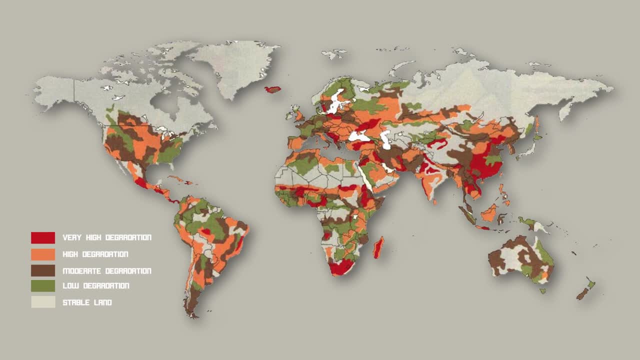 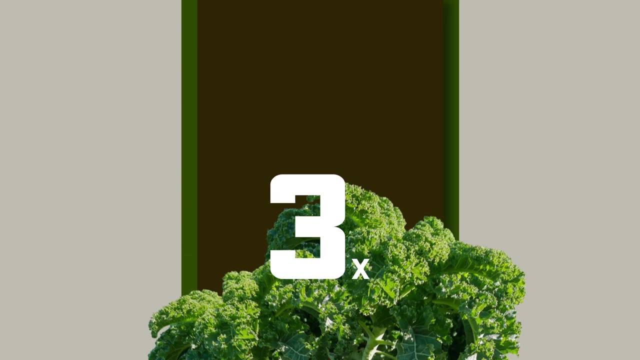 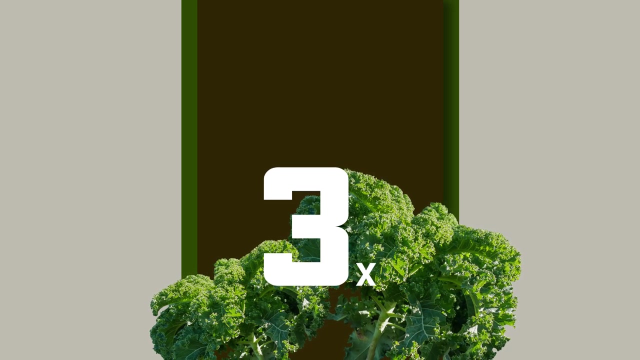 of the world's soil has been moderately or highly degraded, according to the Food and Agriculture Organization of the United Nations, And when you consider that soil can store almost three times more carbon than forests and other vegetation, killing it could lead to our inability to mitigate climate change. 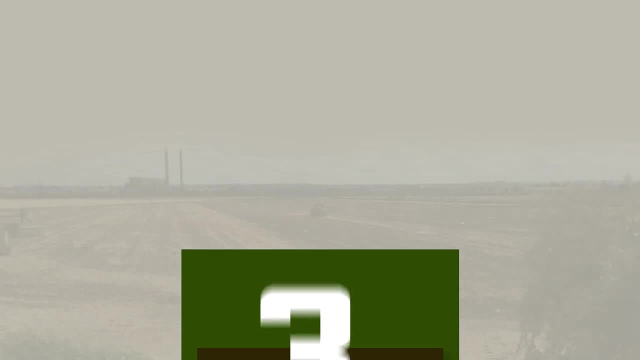 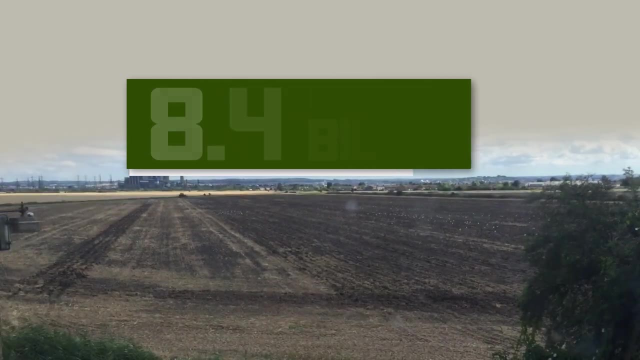 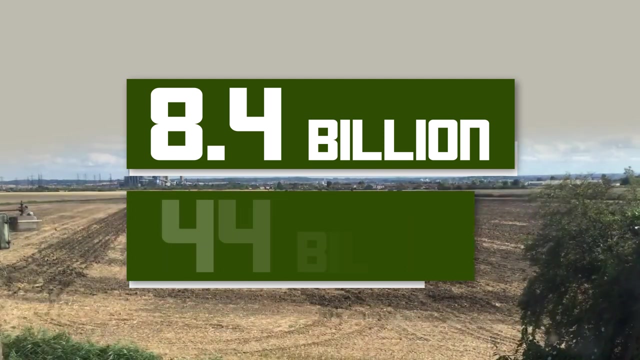 In order to halt this process, we need to reconsider the way we approach agriculture. In Pimentel's study, they argue that the total investment for US erosion control would be about $8.4 billion per year, Considering that erosion causes $44 billion in damages. 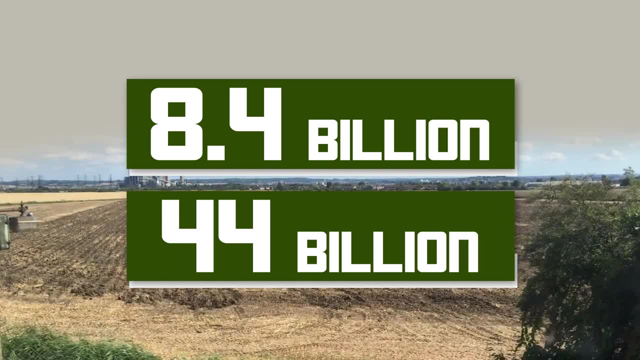 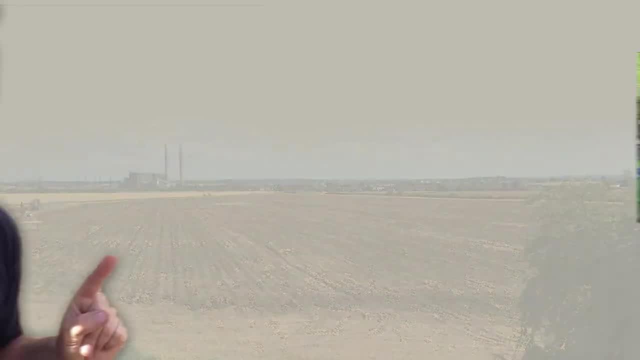 each year and could very well cause more. this is a no-brainer, But on a more basic level, we should look towards the examples of innovators like Curtis Stone, who was able to create a comfortable lifestyle on a low-till intensive urban farm- His farm. 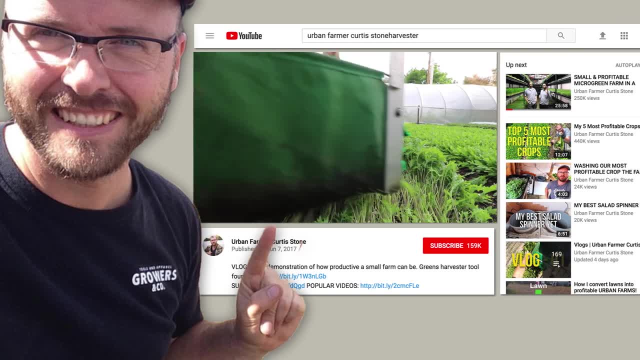 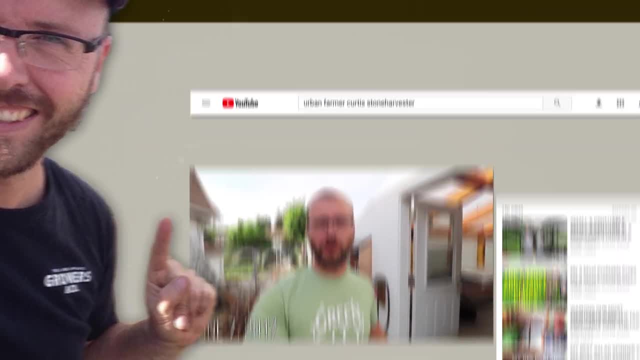 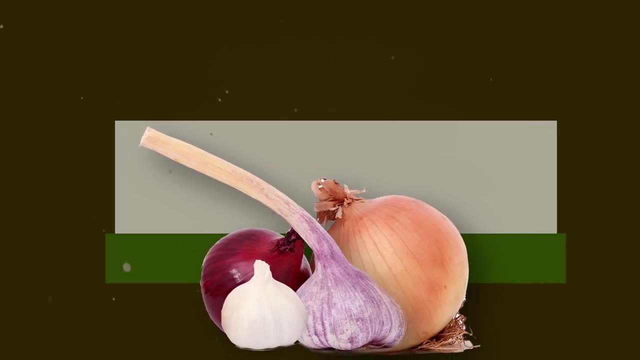 builds soil health by adding compost and natural fertilizer, like turkey manure, to the soil, as well as keeping the cultivation of the land to a minimum. Yes, industrial agricultural practices have provided a large amount of food to North America, But when we consider the long-term negative effects of those practices and the fact that 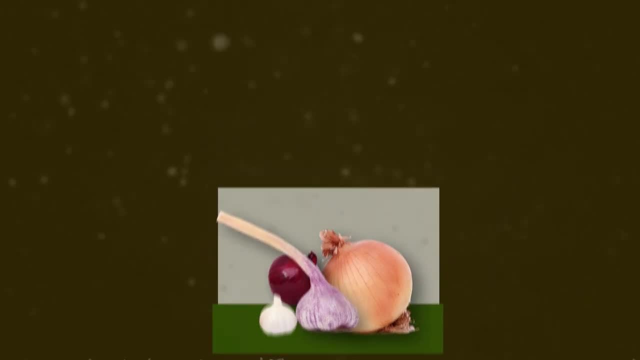 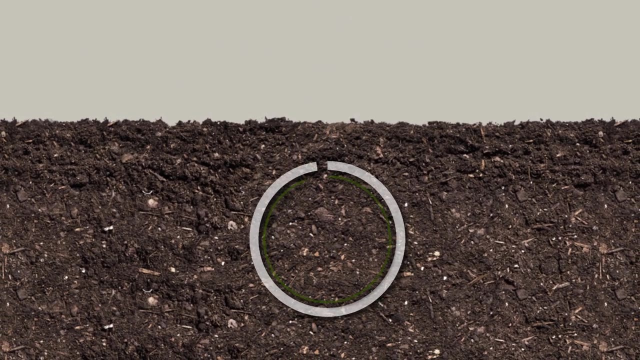 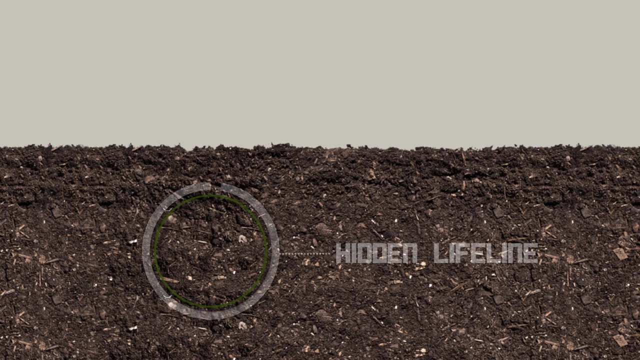 our food system now relies heavily on just a few crops. we can't really say that it's going to make a difference. Positives of supposed abundance merely seem like a flimsy patch for a leaking ship. Soil is our hidden lifeline, and if we destroy it, we lose our ability to feed ourselves.